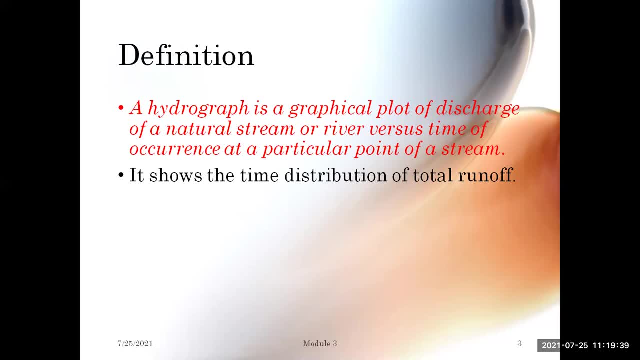 here. so this hydrograph shows the time distribution of a total runoff. So, basically, so, whatever the hydrograph you know which we are going to obtain, so that hydrograph will show the total runoff value, And here the discharge is expressed in terms of cumecs, or hectare meter per day. 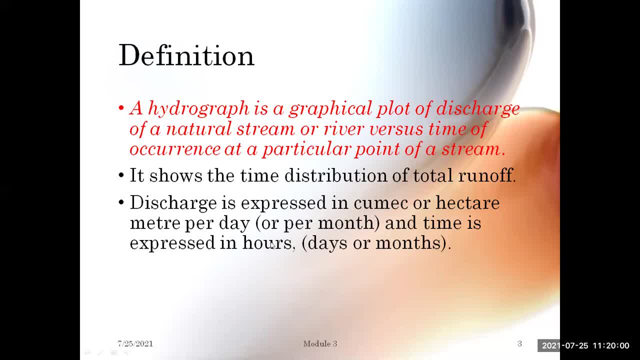 or hectare meter per month, and so time is expressed. the x-axis is in time and y-axis is in discharge, So that is expressed in terms of hours or days or month, And here, so as I have already told, discharge is plotted on y-axis and the corresponding time is plotted. 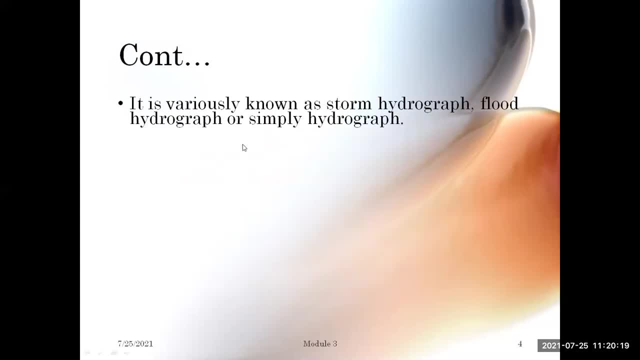 on x-axis, So the hydrograph. so it's called as the storm hydrograph. So we have various names for this hydrograph, So it varies variously known as storm hydrograph, flood hydrograph or a simply hydrograph. So why this hydrograph is necessary? See the detailed analysis of flood hydrograph. 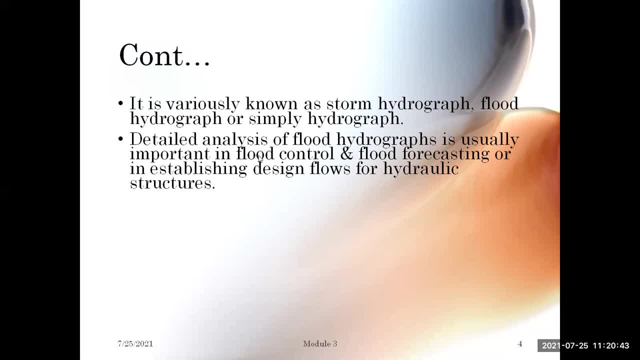 so is very important in case of the flood control and the flood forecasting or, if you want to, you know, establish some of the design. We use hydroids for flood, Dolomites for Crisp, principalmente because the الاavoirmonswsoal and were cleaned. for vocêk大 positions. Hydrographs are generated from runoff which is occurring due to the precipitation, that is, either from a single storm or series of the storm, or would be called storm hydrographs. so whatever the hydrograph, So which represents the runoff due to the precipitation. 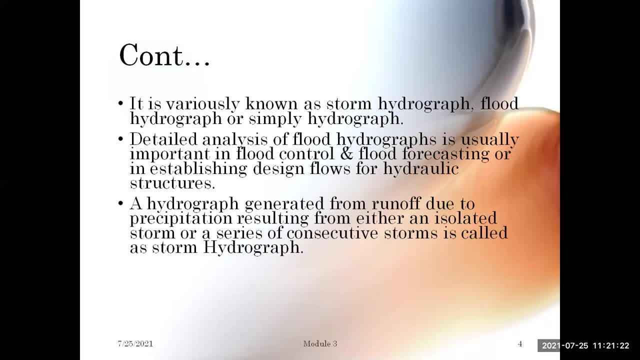 For example, today alone, so which is in times of in surfaces like the flash water. so, for example, precipitation which results from a single storm or a series of storm, is said to be a storm hydrograph, and so hydrograph which is resulting from a single height, storm. that is nothing but. 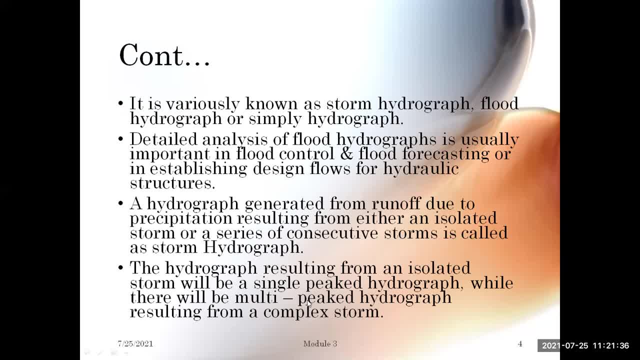 isolated storm is nothing but a single storm, so we'll have only single peak. okay, and also, so if- uh, i know, if- the hydrograph is resulting from an n number of like series of storms, then you will be having a multiple storm. so a typical hydrograph will look like this, so you will be having discharge. 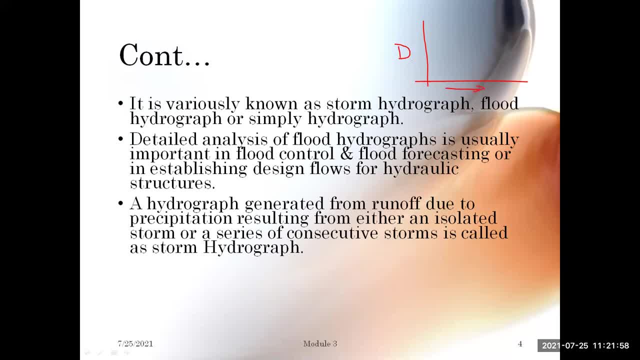 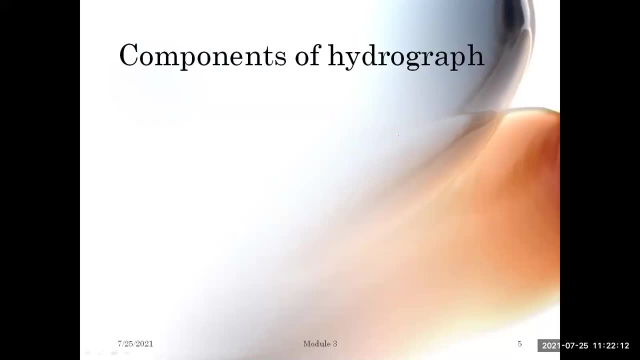 values on the y-axis and on the x-axis. you will be having a time and the graph you're going to obtain like this. so this is a typical hydrograph, and the next topic is the components of hydrograph. so what are the components of hydrograph? see, we have basically 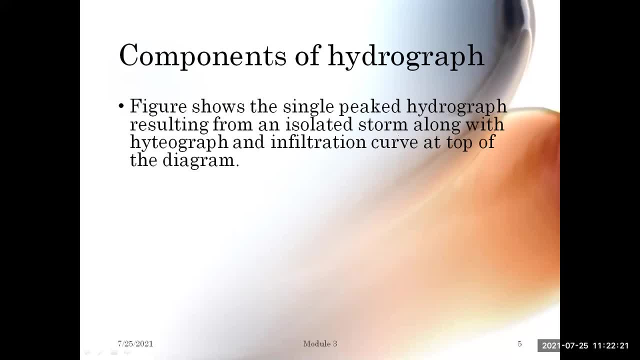 a three uh components of hydrograph. one is the rising limb and the crest part and the recession. so basically, uh, you know, whatever the components which you're going to explain, so that are taken from a single peak hydrograph. so the figure which i've showed in the previous slide, 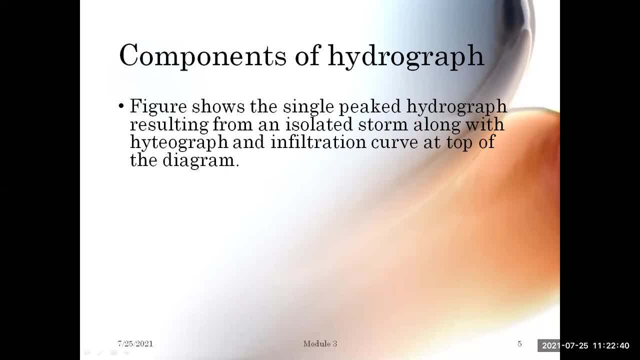 okay, so from a single peak hydrograph. so we have take, which is results from a isolated storm. so we have uh various, uh you know, components. that is that there are three main uh components of the isolated storm. that is called the rising limb and the peak or a crest element, and after that there is the challenge. so these are the three parts of 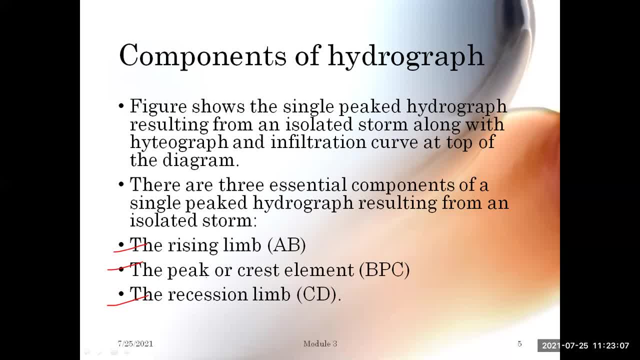 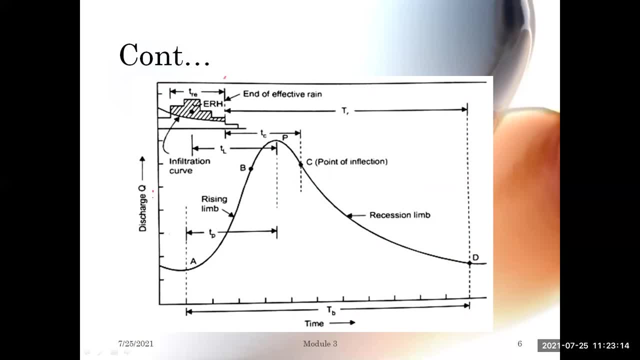 hydrograph. so let us see one by one in detail. what are these components? so the first, uh, you can see the figure here how the typical hydrograph will look like. you can see here: y-axis represent discharge value, x axis represents the time, and you can see the curve here. so this curve is called. 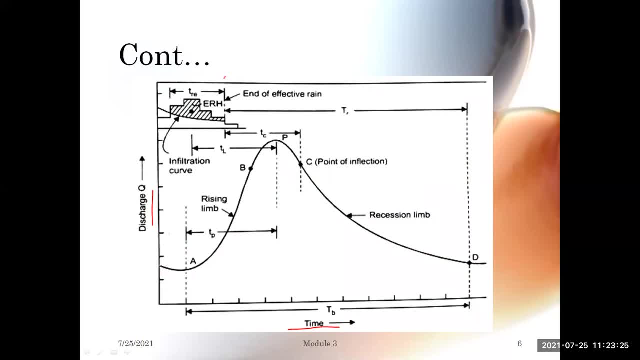 the hydrograph, which represent discharge versus time, and here you can see this particular part, is called the rising limb. the first component, that is e, a, b, is called the rising limb, and you can see here this particular part that is p, c is called the crest part and from c to d, this is called 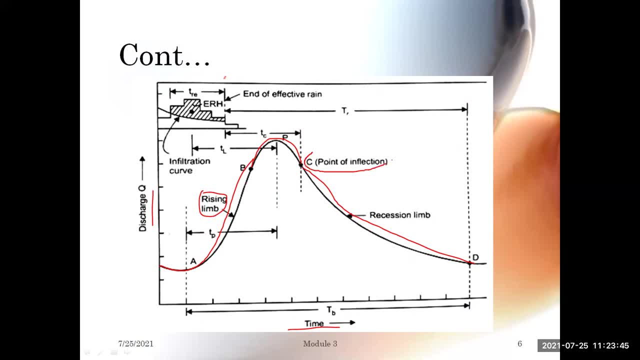 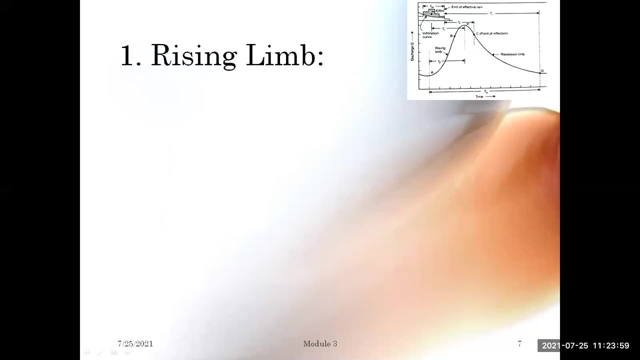 the recession lip. so these are the three components of the hydrograph. so let us see what is rising limb, what is the crest part- and here the point of inflection is there, so that also we'll see- and what is recession. so the first component is a rising limb, that is, the left hand side part, that 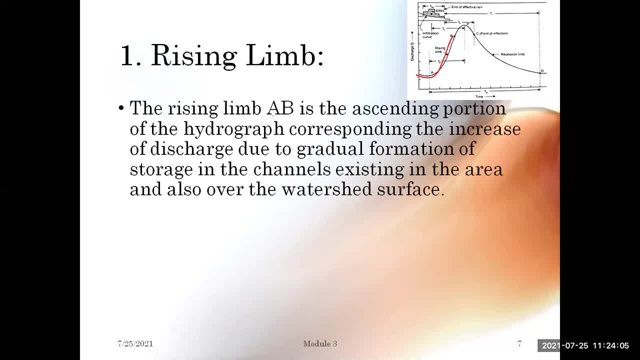 is a, a, b. okay, so the rising limb, a, b is the ascending portion of a hydrograph. see, this is the ascending portion of hydrograph, which is corresponding the increase of discharge due to the gradual formation of storage in the channel, so which is existing in the area and also over the watershed surface. 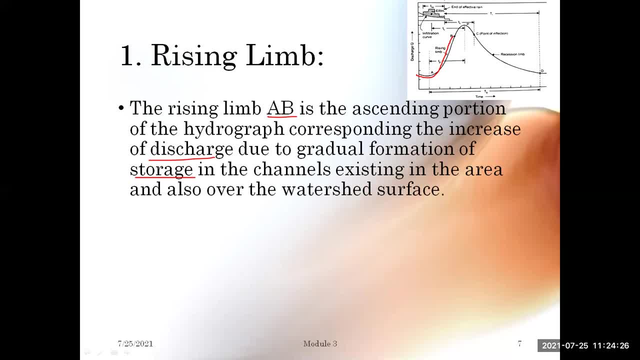 so how this rising limb will arise. this will form so because of the accumulation of the storage. once the storage starts increasing, then obviously the discharge will start increasing. so once the discharge starts increasing, the curve will start rising like this. so that particular part is the rising limb. so this is the rising limb, and this is the rising limb, and this is the. 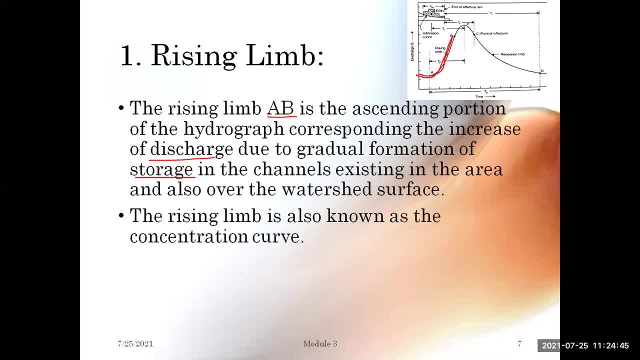 rising limb is called the rising limb of a hydrograph and here it is also known as the concentration curve. the rising limb is also known as the concentration limb and uh. so in the earlier periods of storm there are initial losses as well as high infiltration losses. hence the discharge. 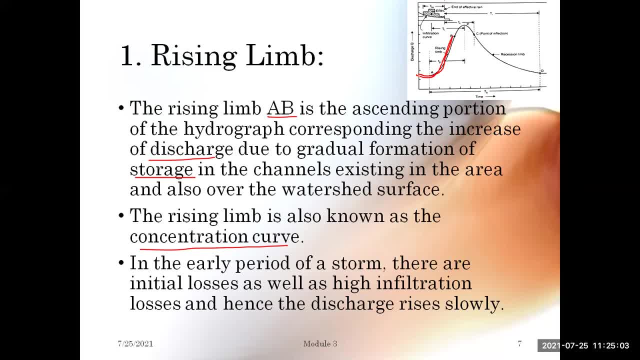 arises. so we see in this rising limb what happened: the rise of a curve. okay, the rise of discharge is very slow because what happens? so at the initial cases, like the less increases year, initially, when precipitation occurs, okay, so there will be a initial losses, that is, you know, infiltration losses, will be gave. so because of that, you know, the rising in storage. 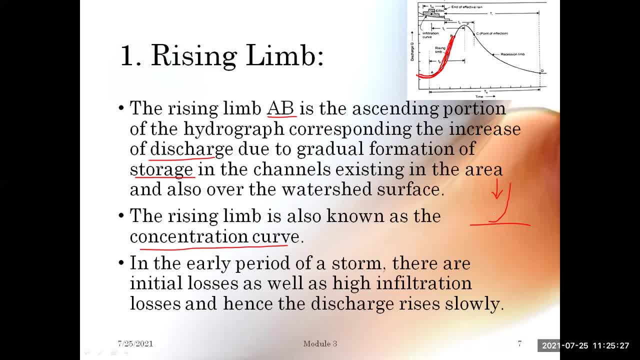 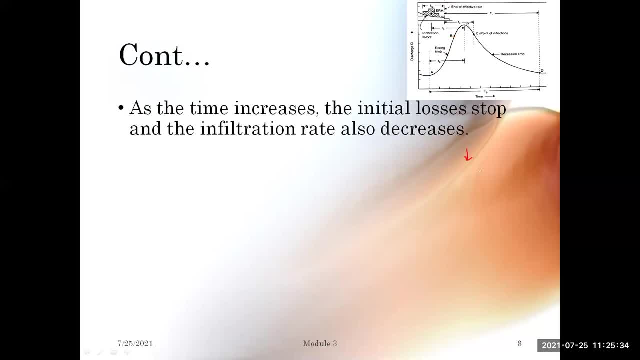 will occur very slowly at the initial stages because of the loss, and also as the time increases, the loss will stop. obviously, as the time increases, as the time of precipitation increases, then what happens? the loses will become less, and so this brings up a quick expectation that, uh, there may be some changes in his maximumなら, into nature. that will come, but just in. case of of of fish andiling which occurs, theaint falei, theеняmusic Drew and ahh faith that ah will have very bad energy, elas of fire and the addictive termination situation which Dor will bring the Grüianid number of dua. so you can certainly visit insects any type of dollars- will become. 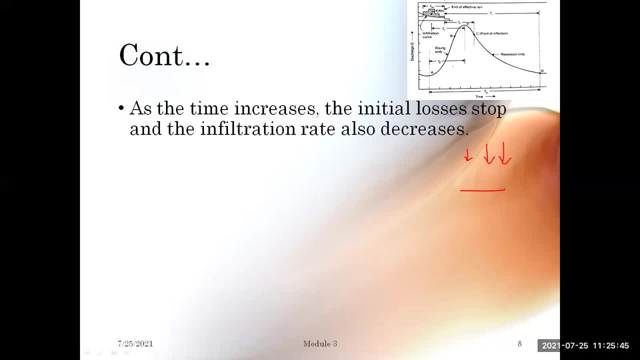 and also the limb will rise faster. okay, The storage is going to increase this as the loss goes on to increase this And, due to that, more and more discharge from the distant part reach to the basin outlet. So, as I have already mentioned, 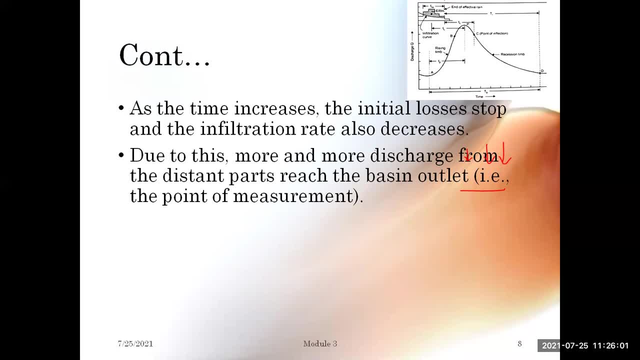 so because of the decrease of losses, what happens? So the storage or the discharge is going to increase. And point A- you can see here from the figure: this is the point A which is called the starting point, So while B is called the point of inflection. okay, 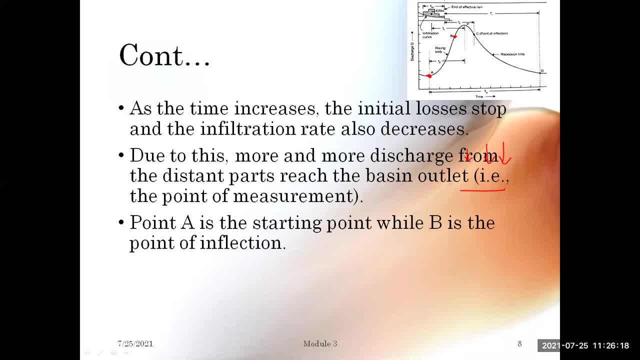 So the curve AB represents the rising limb. So what is that point of inflection means? So that is a point where the curve of the, the slope of the curve, the slope of this particular hydrograph, will become steeper. Okay, that particular point is called the point of inflection. 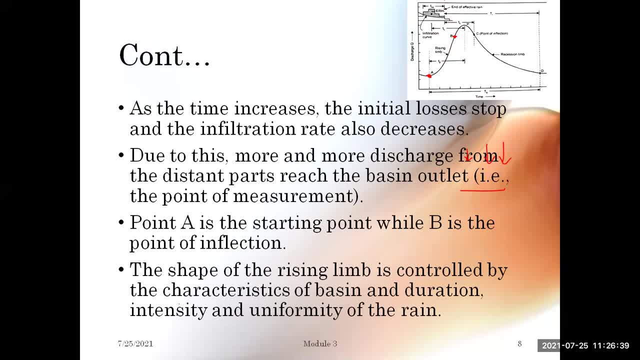 And also the shape of the rising limb is controlled basically by the characteristics of the basin And the duration, intensity and uniformity of the rain. So these are the factors which affect the shape of this rising limb. okay, So that is one is the characteristics of the basin. 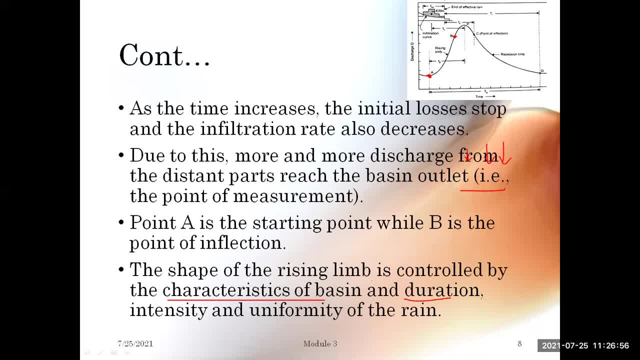 duration of the rainfall and what is the intensity of rainfall and whether rainfall is uniformly distributed. So based on that factors, the shape will vary. So that is all about the rising limb. The second component is a peak or a crest segment. 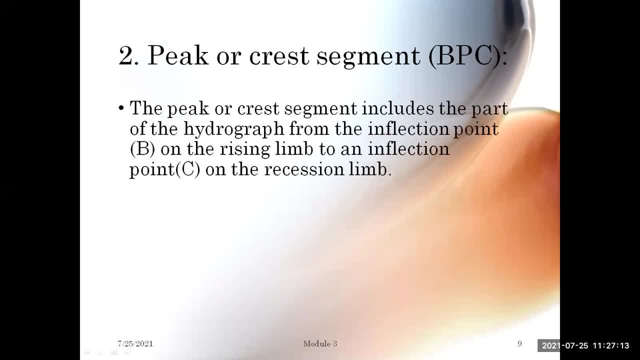 which is the peak. This is called PPC, So as you see in the figure, So the peak or crest segment includes the part of hydrograph. So from the point of inflection, that is, from B on the rising limb, to the inflection point on C, 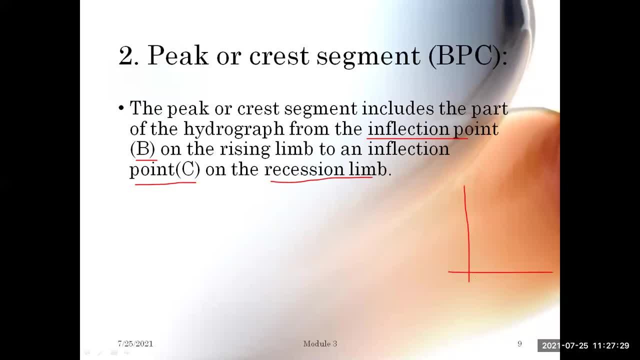 which is on the recession limb, for example. So if you consider, this is the you know curve. So here there was a point B, and this was point A, So B from the point of inflection on the rising limb and the point of inflection on the decision curve. 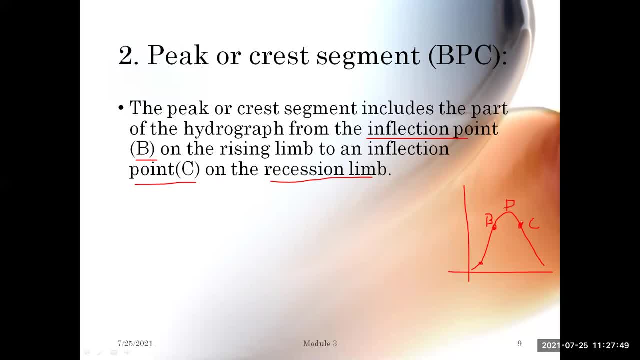 So this particular part, so this is a, B, So this segment is called the crest or a peak of the hydrograph. So this, both B and C, are the point of inflection. So B is a point of inflection on the rising curve. 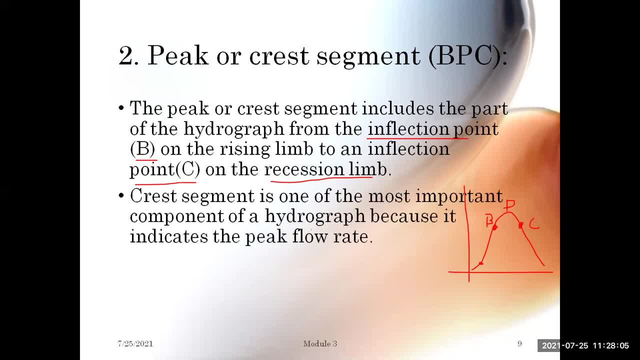 and the C is the point of inflection on the recession limb And the crest segment is one of the most important component of hydrograph because it indicates a peak flow rate. so because as this indicates the maximum flow rate, so this is very important because we are 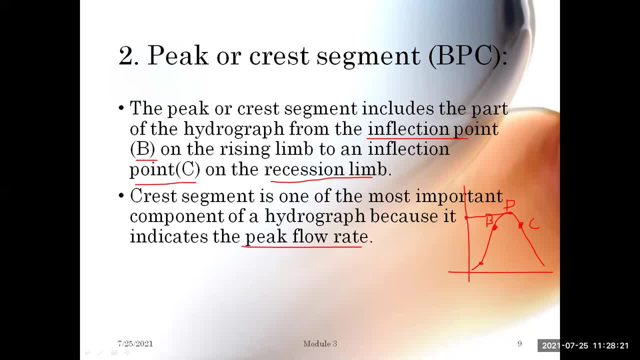 going to whenever we are going to design a hydraulic structure or whenever you are going to do a flood hydrograph analysis. so we are going to take the maximum peak flow and the peak represents the arrival of flow at the outlet from all parts of the pacing. so this, whatever this, 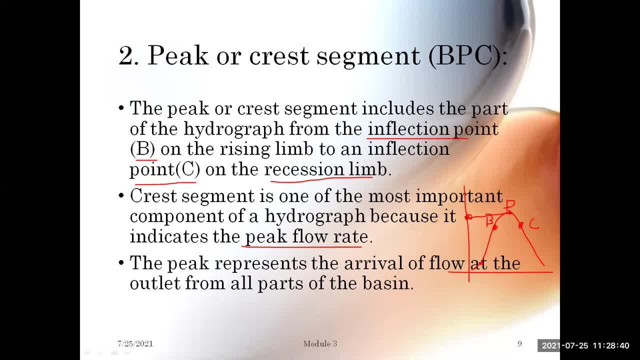 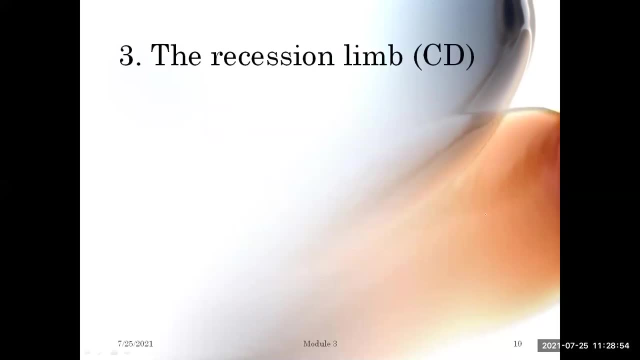 peak represents. so the peak point represents the arrival of flow at the outlet from all the parts of the basin. okay, so this represents so the flow of water from all the parts of basin. and the last component is the recession limb, which is called the cd. okay, the recession limb extends from the 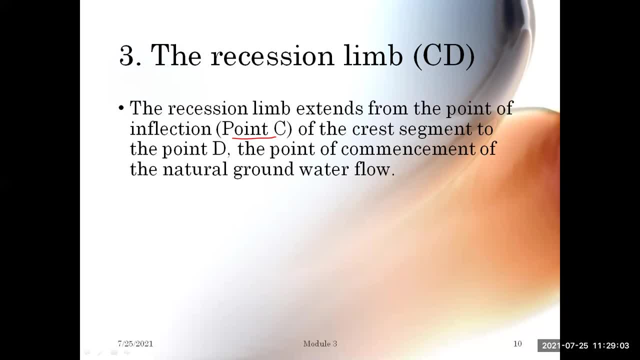 point of infection, that is, from point c of the crest segment to the point d. okay, so i think this particular part, you can see this is the d or in the graph and this is the point c in the curve. okay, so this from c to d. that is point of infection to last. 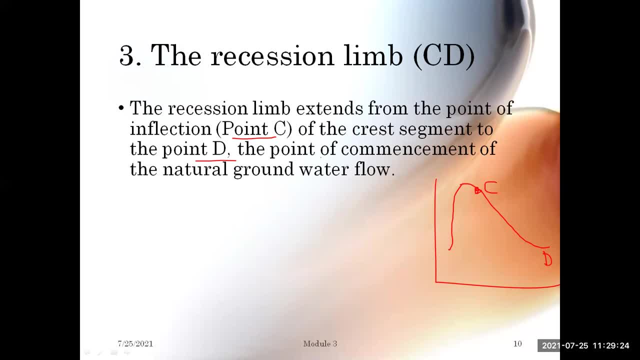 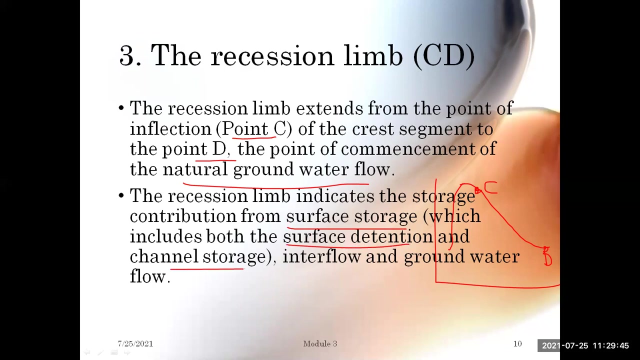 crust, segment d is called the recession and this is the point of commencement of natural groundwater flow. so this point d represents the commencement of groundwater flow and the recession limb indicates the storage contribution from the surface storage, which includes both surface retention and the channel storage, so an interflow ground water flow. 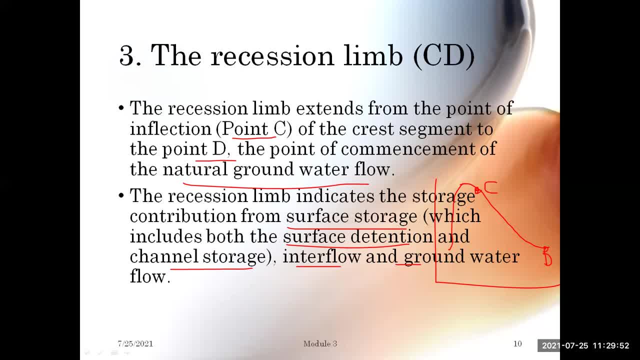 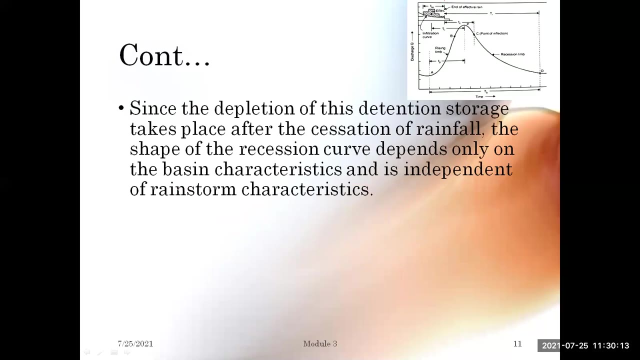 okay, so whatever this uh, you know the recession, limb, uh indicates, so recession, them, cd indicates the storage from various surfaces, like you know: surface retention, interflow, ground water flow, so all those included in this precision and limb part. so that is the third component and also so since the depletion of this detention. 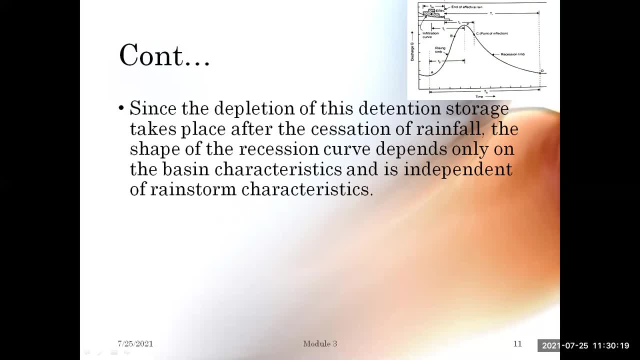 storage takes place after the session of rainfall. the shape of the recession curve depends only on the basin characteristic and is independent of the rainstorm characteristics. see what happens. whatever this retention storage is that they see today, this particular part represents the- uh, like the storage and detention storage- groundwater flow, internal flow, which occurs below the ground. 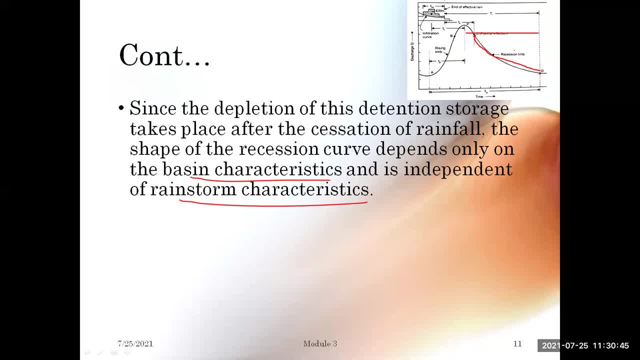 surface. so hence this does not vary with respect to rain characteristics. it will vary only with respect to the base in characteristics. so that is the one important part in the decision curve, and it can be considered as a rate of discharge resulting from a draining of process. like you, 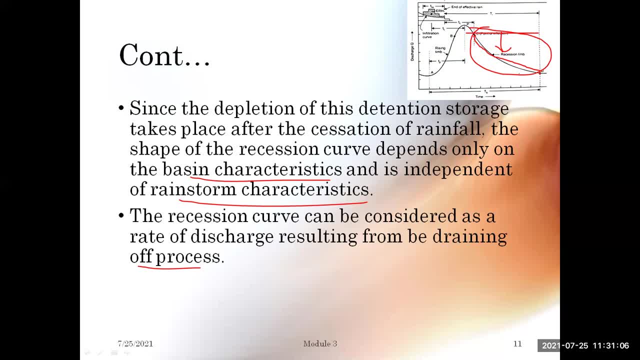 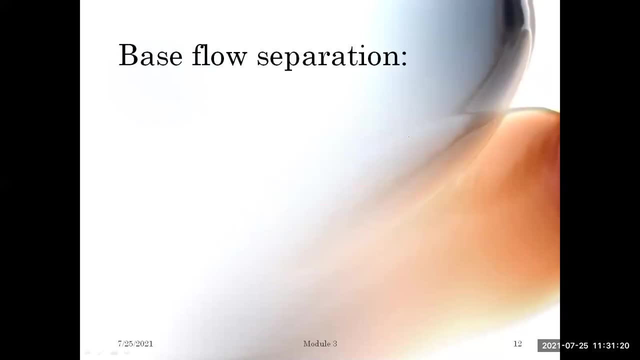 know, groundwater flow, interrupt flow- all those are called the trainees- and rain flow between the flow, those are called the training process. so, whatever the curve which is results from the draining process, that is called the recession curve. so these are the three components of the hydrograph. so the next topic: you have the base flow separation. so basically, uh, you know, 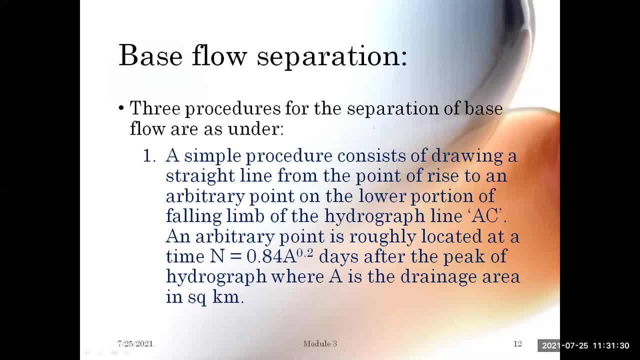 we have three methods to separate a base flow from the total runoff. so the very first method uh is: uh, you know, the simple procedure, like you know, consists of drawing the straight line. so from the point of rise to an arbitrary point on the lower portion of the falling limb, on the hydrograph line, 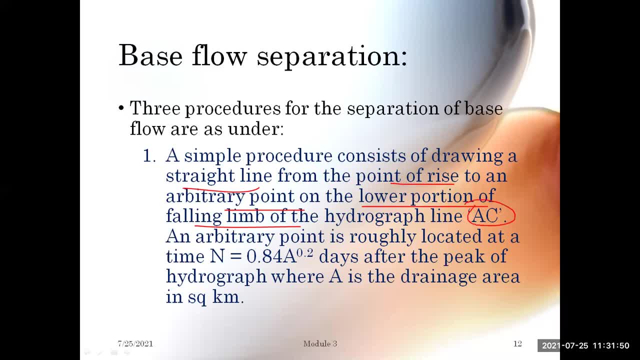 so, which is denoted as aac. so, and an arbitrary point is roughly located at a time. n is equal to 0.84 into a to the power: 0.2 days. wherein represents the number of days after the peak of hydrograph. so when 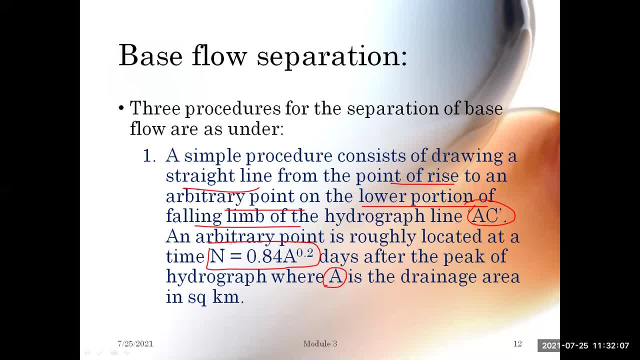 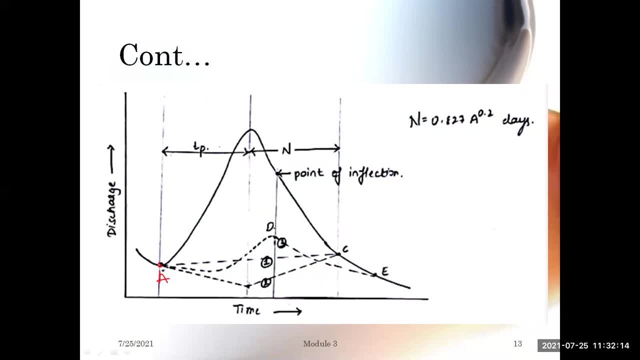 a represents the drainage area in a kilometer square. so if you see the figure here, you can see here that this particular point is the point of price. so the first method is: so you have to draw a straight line from the point of rise to an arbitrary point which is c. okay, so where this? 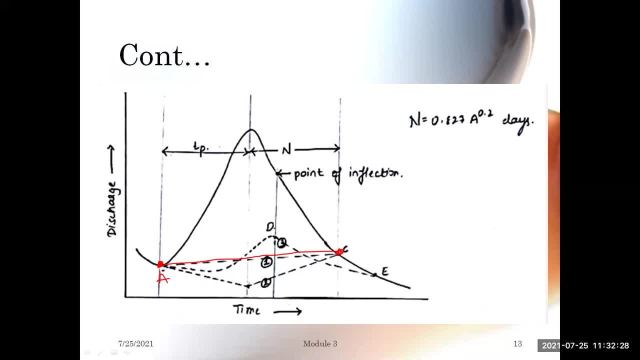 arbitrary point is selected, uh, to be occurring at n number of days from the peak flow. so this arbitrary point c is selected to be at n number of days where n is equal to 0.82 or into a to the power 0.2. so that is where a is the base in area. so this is the first method of base flow separation. 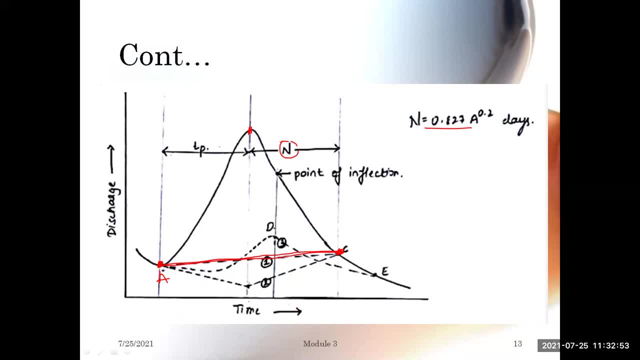 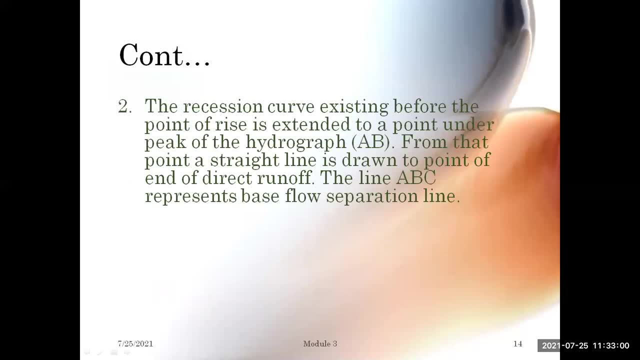 so this line a c represents the base flow separation line. so, similarly, you have the second method. the second method is the decision curve existing before the point of rise, okay, so. OK, the recession curve, which is existing before the point of rise, is extended to a point under the peak of hydrograph, so which is EAB. 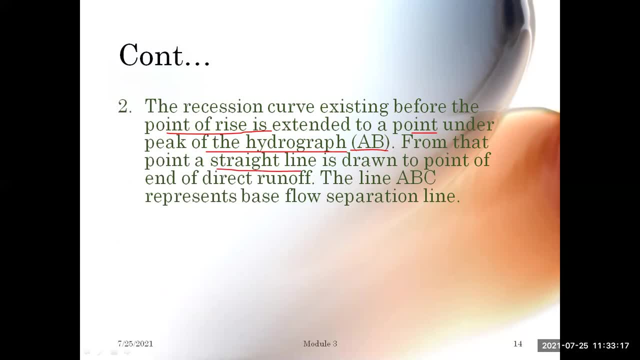 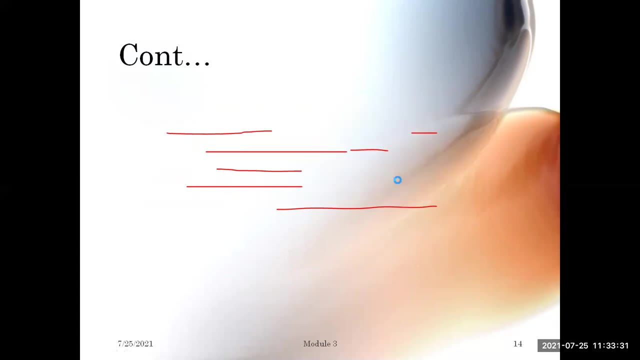 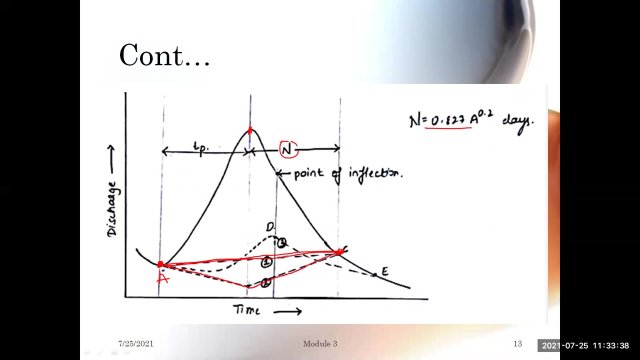 OK, so from that point a straight line is drawn to a point of end of direct runoff. OK, so the line ABC represents the base flow separation line. OK, so, if you see the figure here in this particular part, so the line ABC, see, this is the ABC line so which represents the second method of base flow separation. 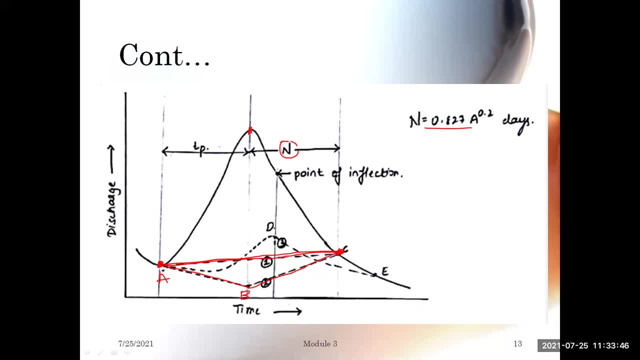 So first, what you have to do is you have to draw a line, EAB. so from the point of rise to a point which you know joins the peak flow. You can see, this is the peak flow. So from the point of rise, 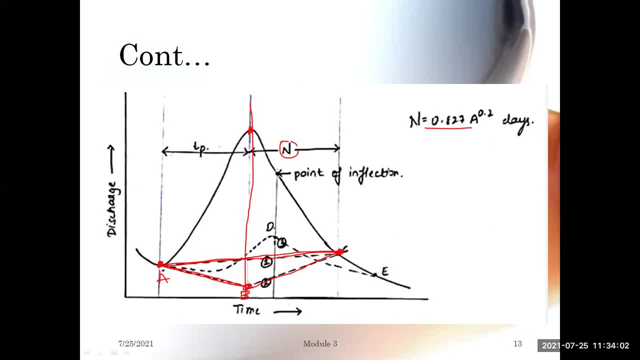 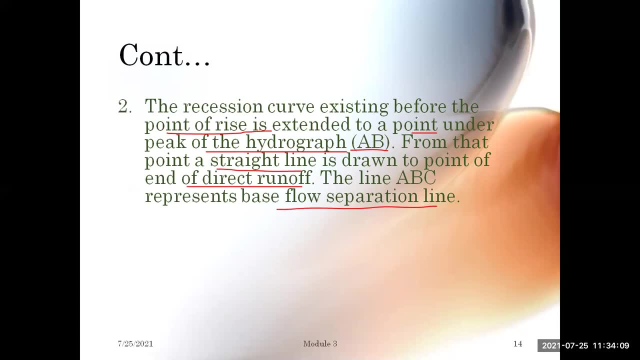 OK, So from the point of rise, So from the point of rise, So you have to draw a line AB which represents the EAB, So where you can see here so the recession curve existing before the point of rise. So you can see here: 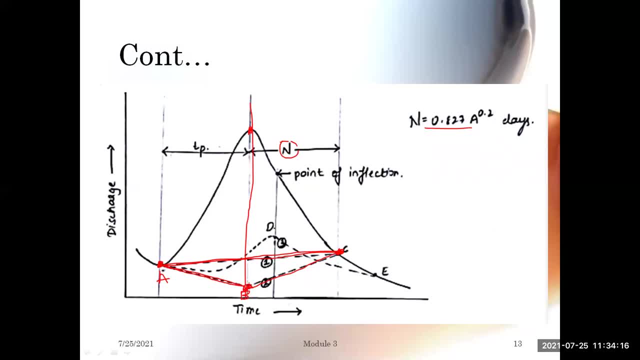 So before the point of rise means. so you can see B is before the point of rise, that is A. So B is before A. So from A you have to draw a line AB and after that. so you have to join this. 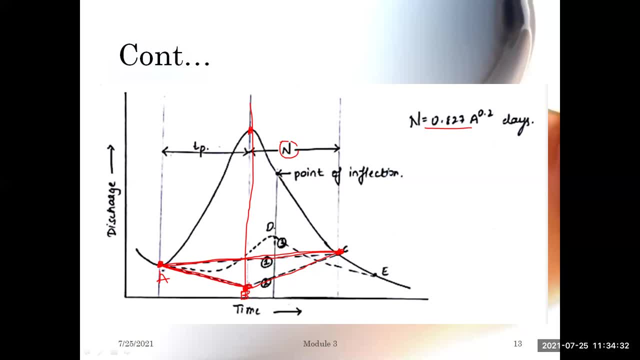 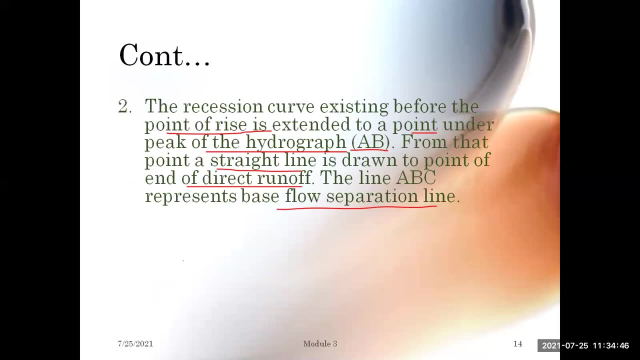 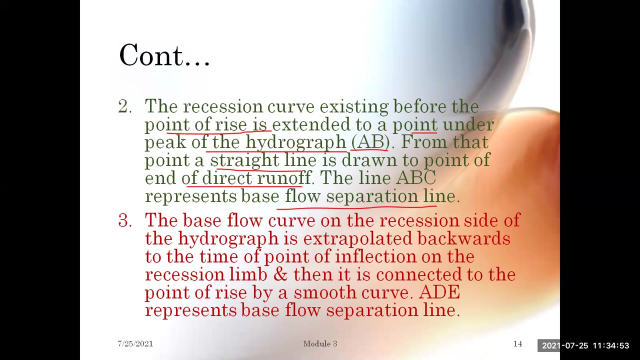 I know the point which which joins the peak flow. So to join an arbitrary point that you see. So where this ABC line represents the base flow separation line from the second method, So the last method, the third method, is this base flow curve on the recession side of the hydrograph is extrapolated backward.